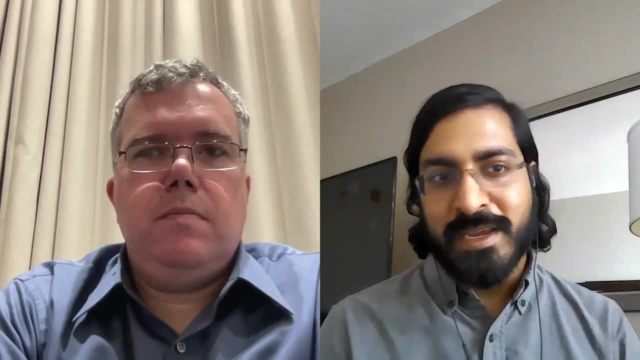 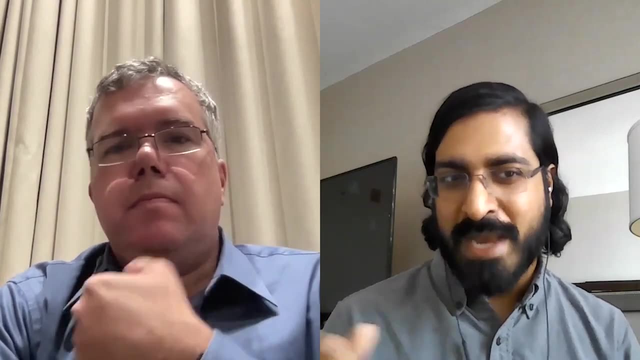 the nature of it. sometimes you're filling in the structure, sometimes you're fitting a particular model, structures, parameters to us to try and produce an output. but the idea is that you have a mathematical representation of kind of everything in the space that you're working with. that's kind. 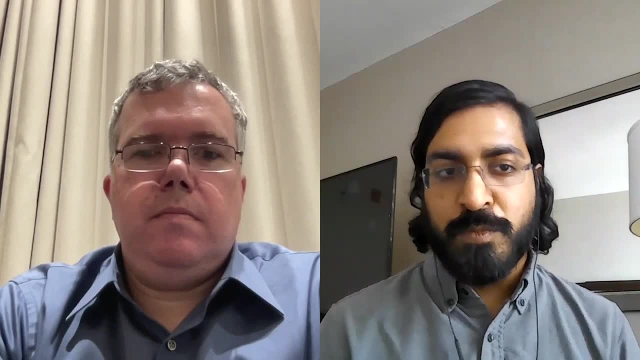 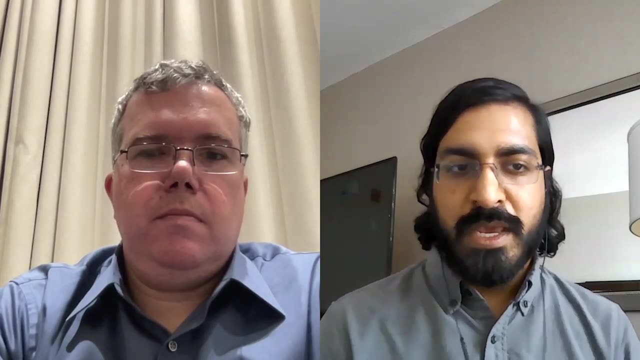 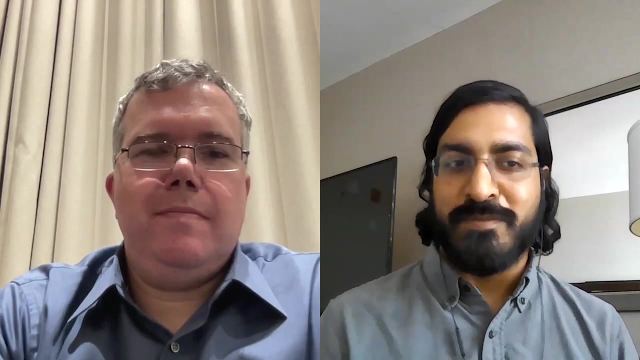 of your framework for doing this. the project I worked on recently with digit is using this new space of of large language models, and so this is a relatively new area where- well, I mean the areas existed for a while, but there's been some very, very impressive upgrades to the technology. 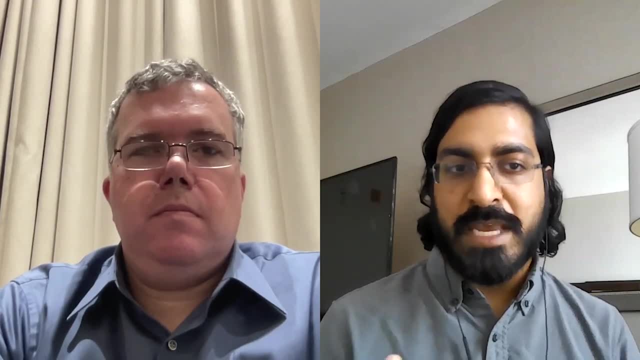 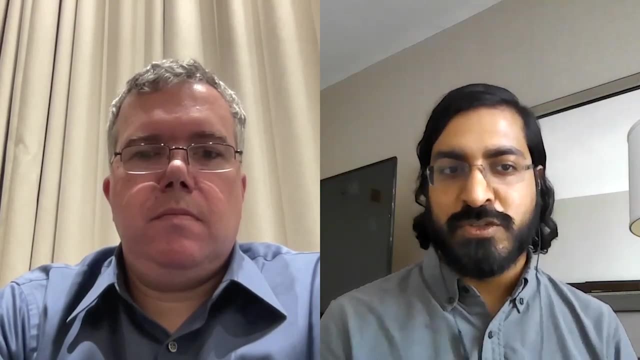 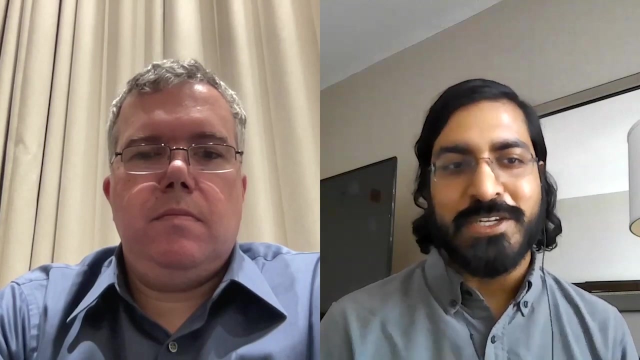 in recent years where it's possible to basically take a model that's not specifically trained on what digits doing or a mathematical framework or any sort of structure around what digits doing. it's instead trained on a very large corpus of data about just things in the world in general: right things humans do, things in human. 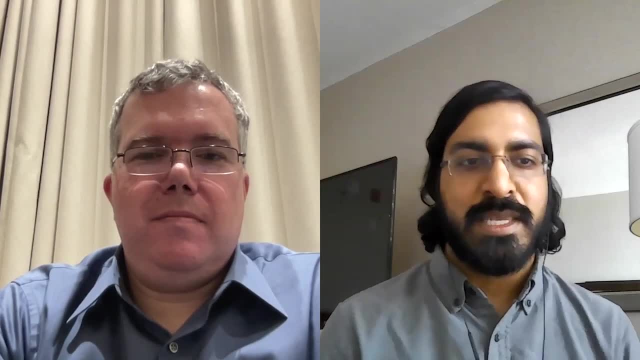 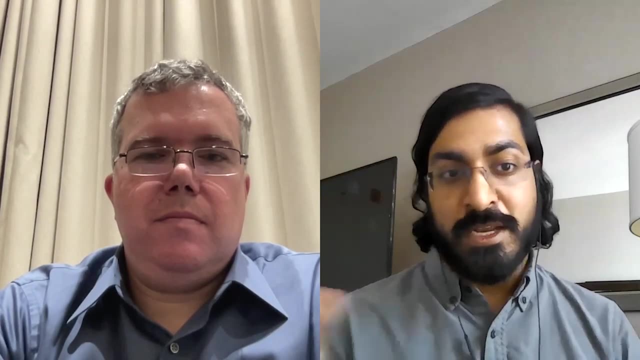 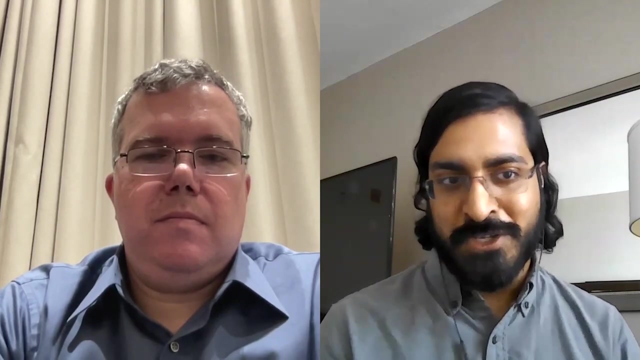 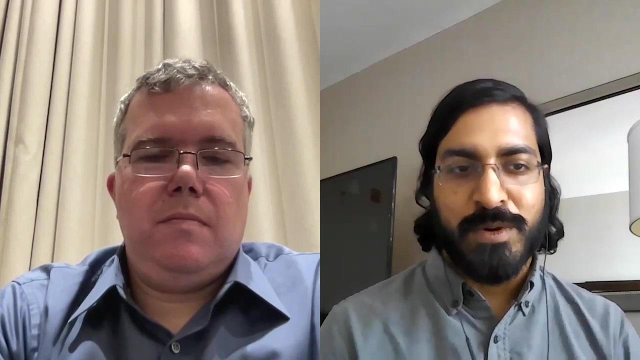 worlds, objects, ideas, semantics and this very large model right, and these are very, very large models, billions of nodes in a huge network to encode this interesting representation of this idea of a general semantic world and you can create queries against this general model of a semantic idea of a world. and if you generate the queries, 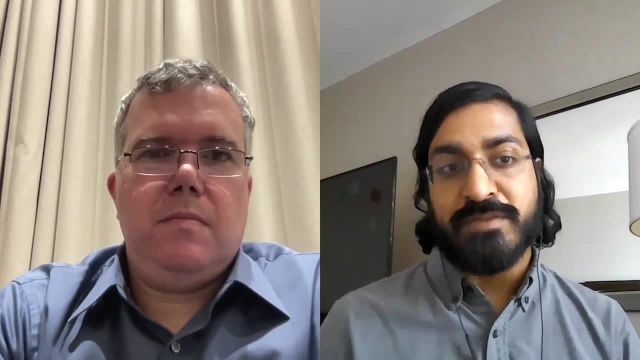 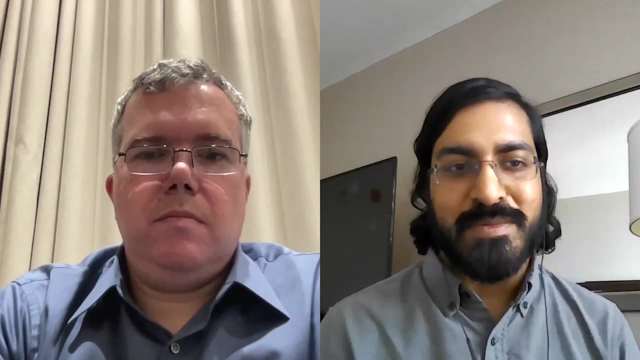 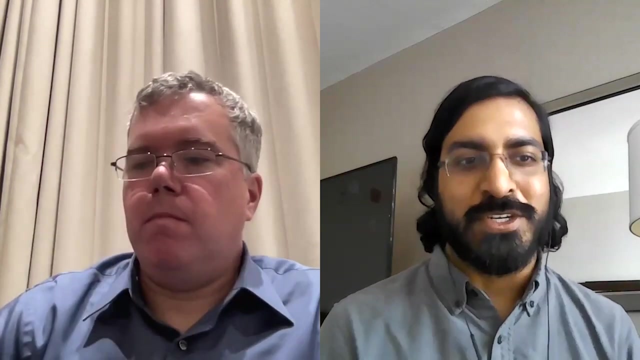 right, then you can have these bottles generate out, you know, a set of tokens which encodes a response, and that's actually a fairly groundbreaking thing like this is even that this is even possible with lms uh, that you can train up a model on a generalized representation of just the world structure and say: and now, if I tell you to complete, 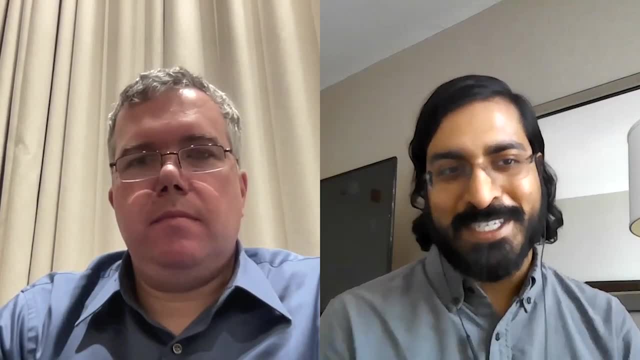 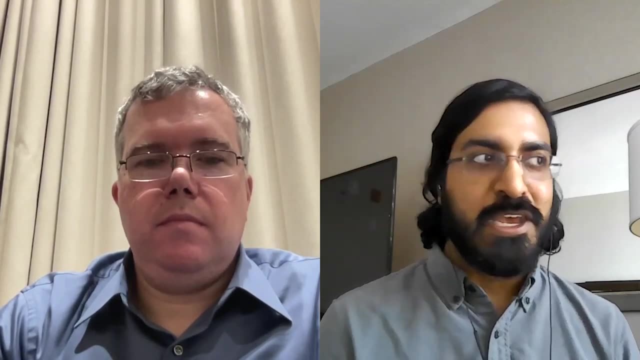 this sentence, where the first part of the sentence is a question and then the second part of the sentence you're going to tell me the answer to that question and for it to not just generate something that's, uh, a sort of list of words that are sort of vaguely related to the question. but 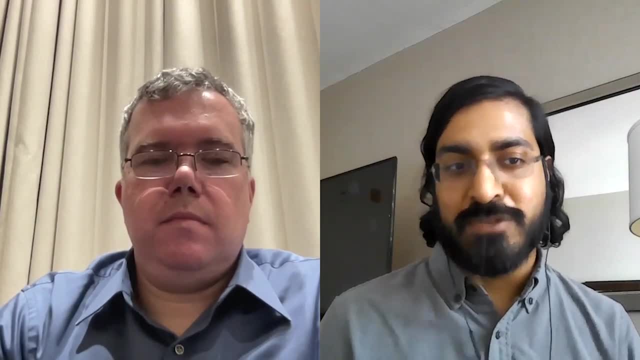 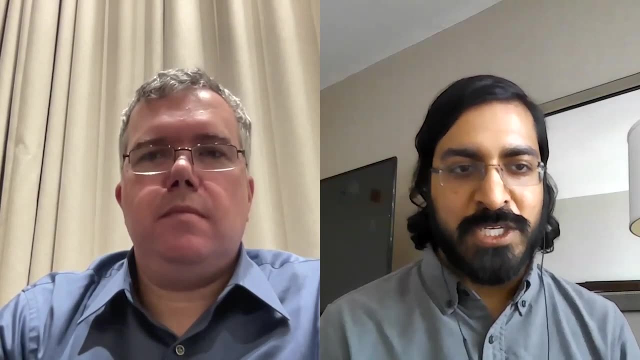 to actually generate something which actually contains knowledge, representation about the purpose that it's been trained on like. I find that amazing that that is something that we've been able to achieve, but now that we have figured out how to do that, obviously there's many caveats to. 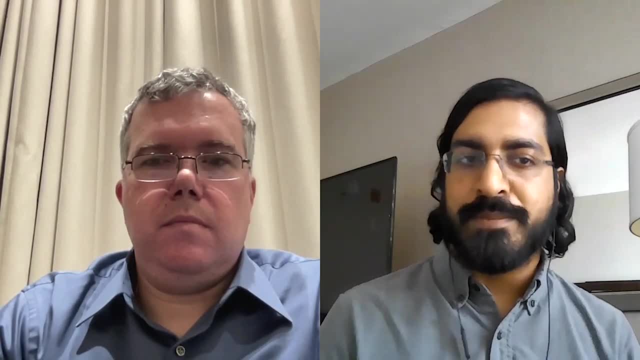 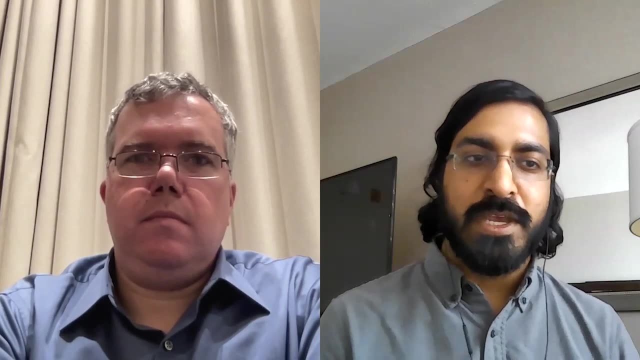 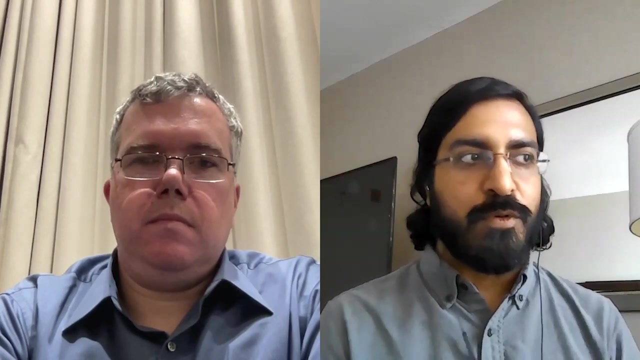 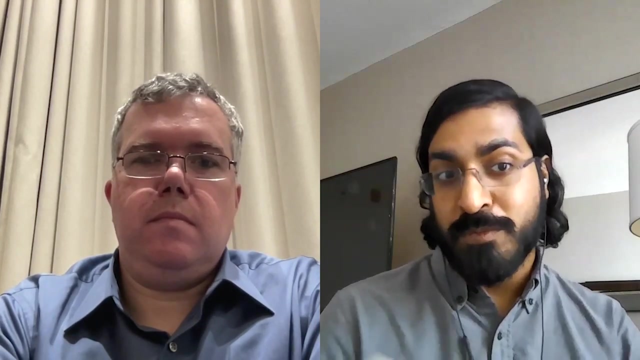 the complexity of those answers. but you can engineer those prompts and you can build upon them to have them form fairly complex generated responses, and so in this case we can form prompts which are going into this llm that are specifically asking or prompting for uh questions about digit. so digit is in this space, digit is seeing these items. what would digit do? 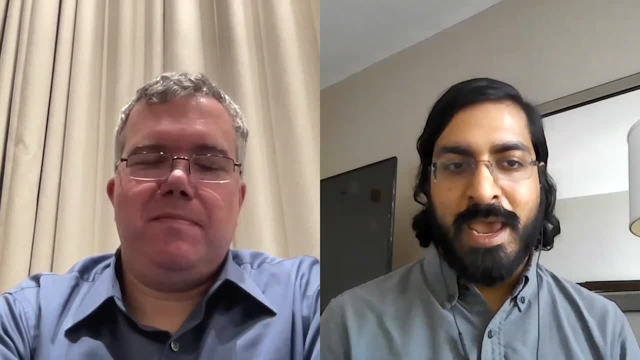 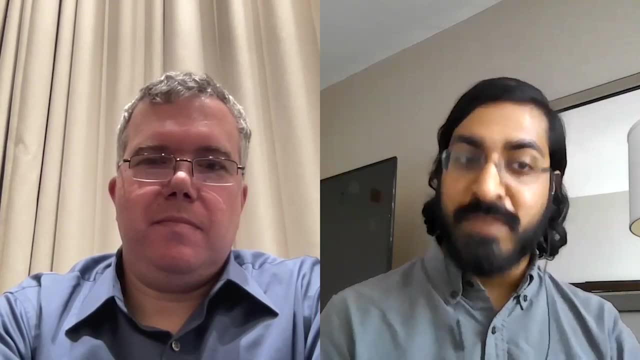 next if it was asked to solve a particular problem, and it'll actually generate a response. and the interesting part is that we can construct that response such that it's in the parlance of things that digit can do, and that's where it gets particularly interesting. you now have the 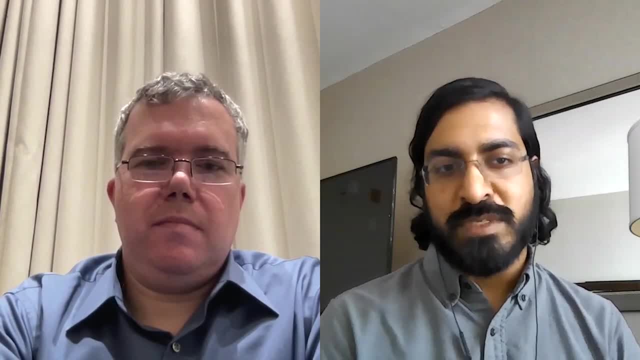 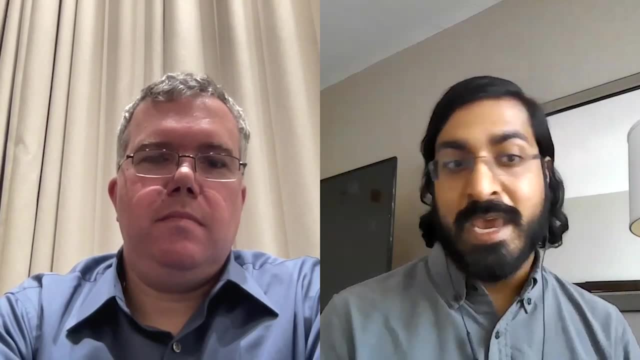 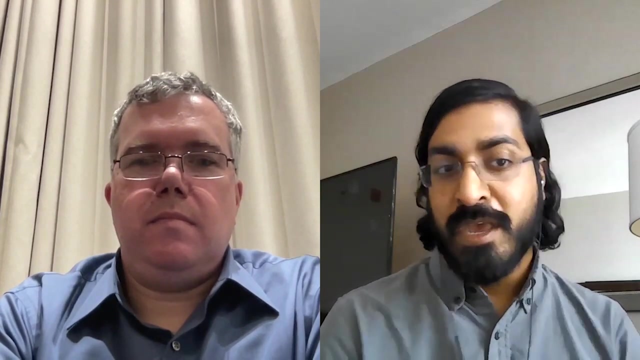 ability to encode the embodiment of digits capabilities again in a form that this, like reasoning engine can understand and it'll produce a response, which is the thing which is out of the set, that of things that digit can do, like picking up objects, moving around an environment, putting objects places, and you know additional stuff, like doing gestures or walking around, if 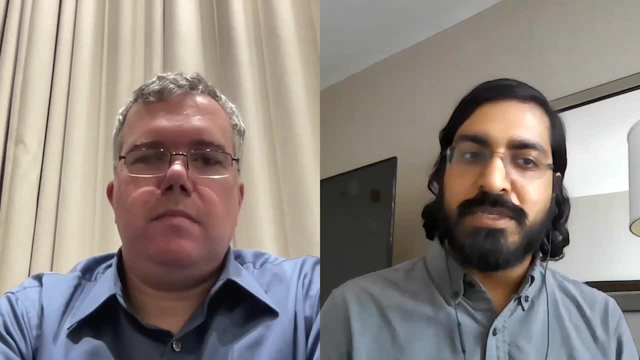 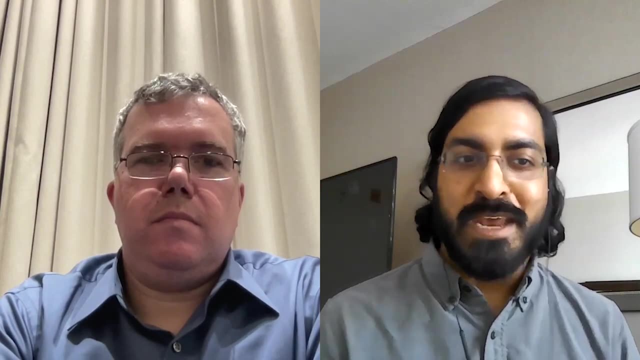 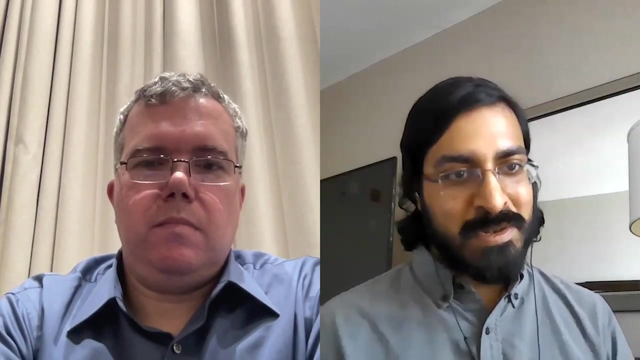 you think that that's helpful to your cause, uh, and it will produce some structured response that can do. you know sequences of these things in various forms and of course now the question becomes: you know what is the right way to harness that? and that's a really new and interesting question. that now 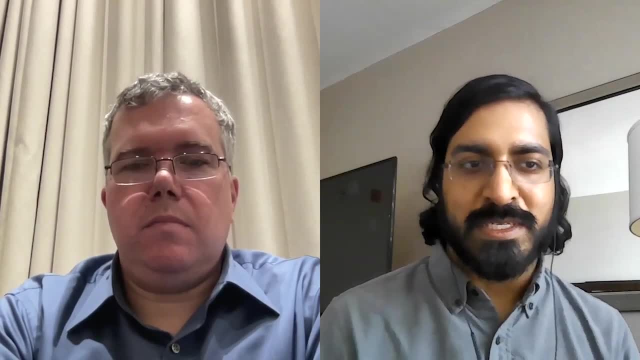 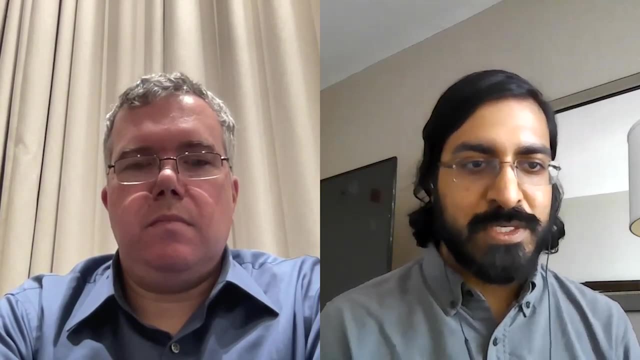 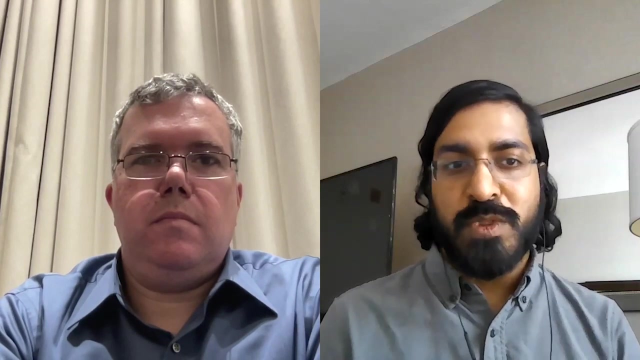 that we have these models available. a lot of people are scrambling to solve, like: what is the right way to encode this question? what is the right way to decipher the results? now? with uh digit in particular, one of the advantages we have is that digit itself both has a very common 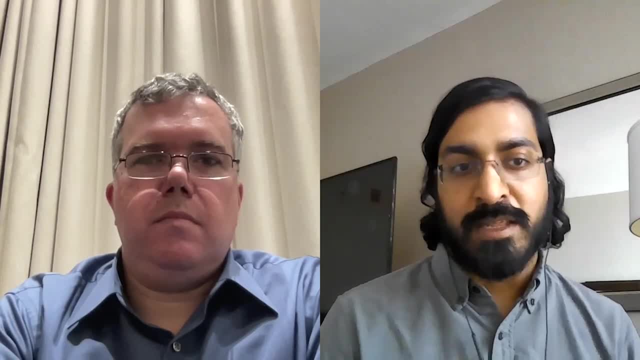 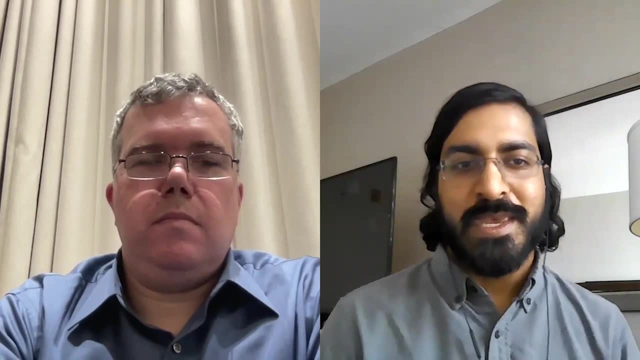 semantic lexicon with the data set that that the llms are trained on. uh, because it is a human-sized, human-scale robot that can operate in human environments. that's the corpus of stuff that that we've been training llms on largely, so we get a lot of value out of that. 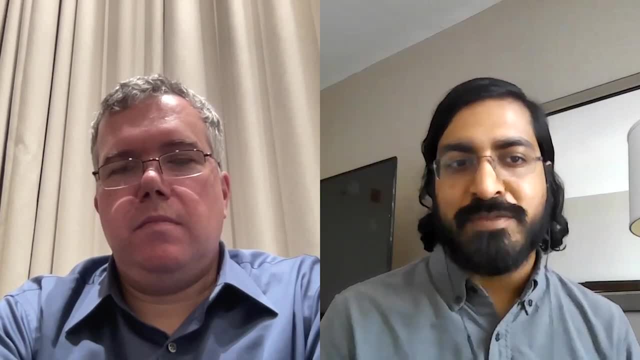 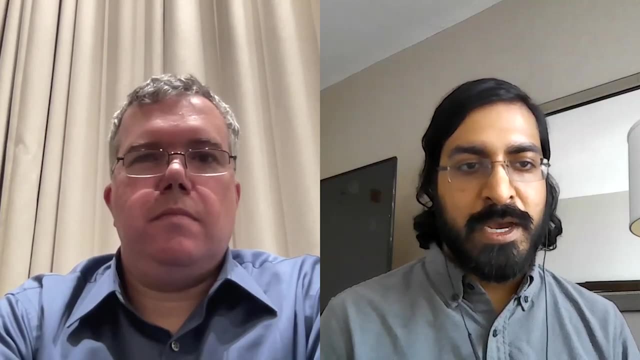 and the second part is we've built digit to have a lot of physical intelligence, to be able to move around and interact in these environments, to be able to exert forces without you know um disrupting human environments, and that means that it can. it can provide a sort of comprehensive